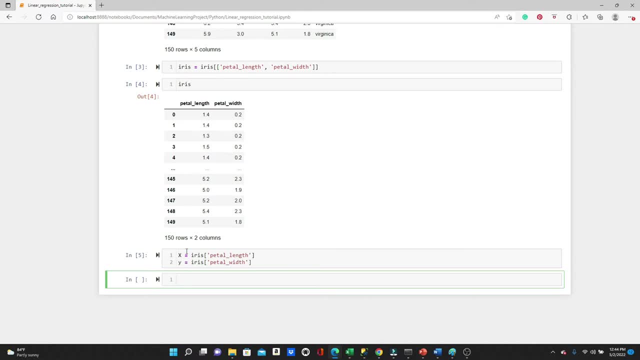 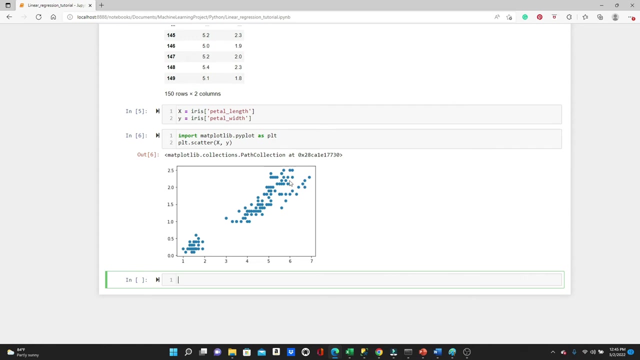 we need to have some relationship, some correlation between x and y to be able to perform a linear regression. So let's see if this x and y have something of correlations. So import x, y and y are the parameters, matplotly dot, pi plot as plt. so plt, dot, scatter x, y. look at it, we actually have some correlations. 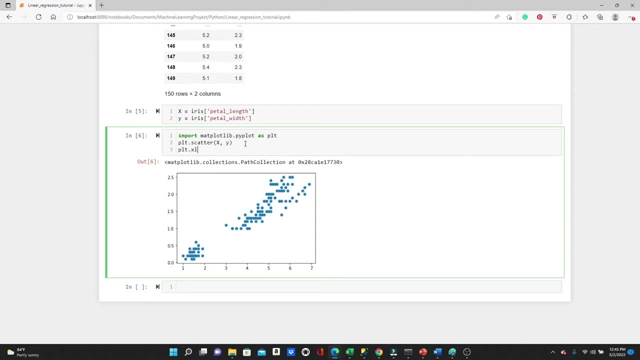 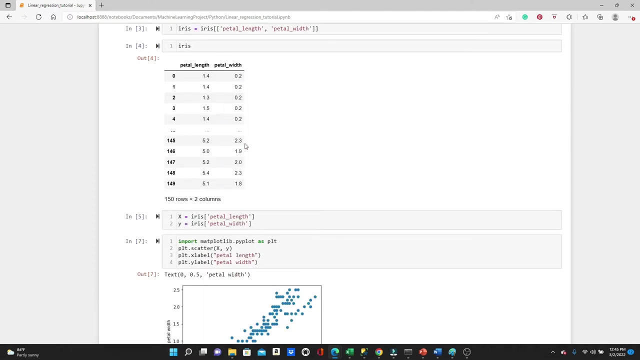 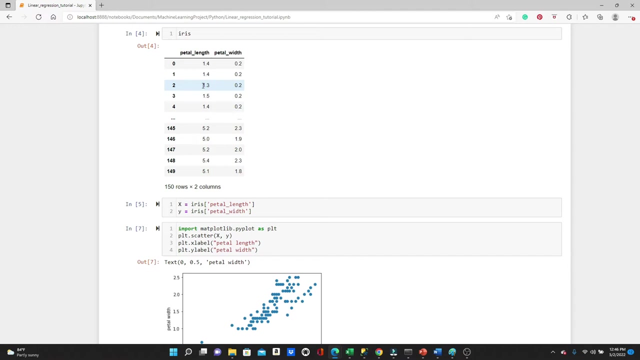 some good, positive correlations: plt dot x label- pedal length and plt dot y label- uh, pale width. before we move on to any machine learning, we usually split the data set into training and test data set, so we can use the training data set for training purpose to train the model, and we 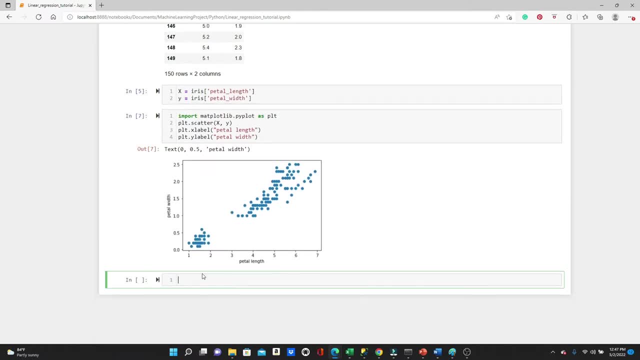 can test the model using the test data set to do the splitting. we have the function train test split. so from sklearn dot model selection, import, train test, split, now x train. do this: x train, x test, y train, y test. then train test split x, y. okay, now we have to give a test. 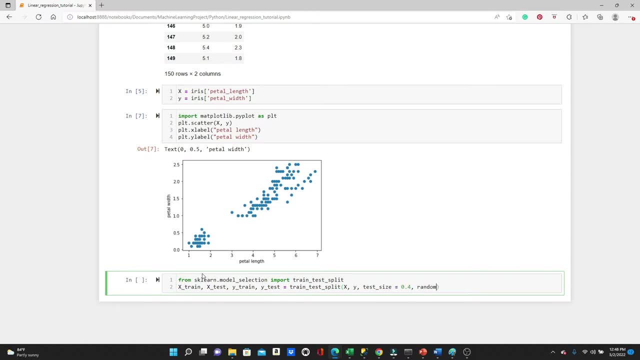 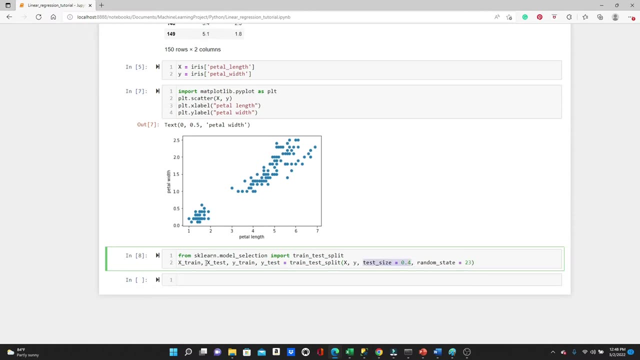 size 0.4 and a random state 23. what test size 0.4 means? it means that it will keep 40 of the data for testing purpose as x test and y test and fly random state 23 for that. let's see x train. look at the x train here. 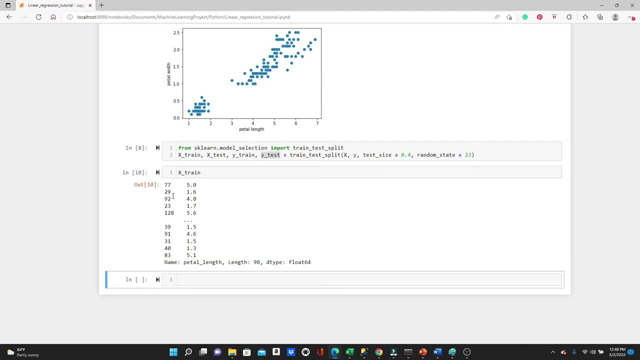 look at this row, number 77, 29, 92, 23, so it takes the random rows. it doesn't take top 60 percent or bottom 60 percent for the training data or top 40 percent or the bottom 40 percent for the testing data. it takes it random rows to make up that 60 percent or 40 percent. if you run this train test. 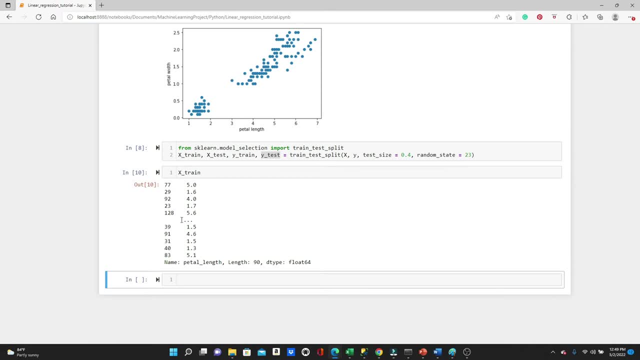 split again, it will take different random rows. so if we want to recreate the same splitting, we have to use a random state. and this 23 is not constant. you can use any other number, but when you regenerate the data you have to use the same number. this is: 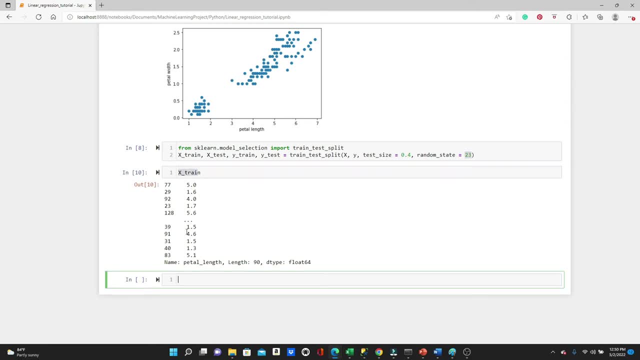 the same step as before. that's how you can do this x train and x test split. then x train is one-dimensional. in psychic libraries the machine learning algorithms take two-dimensional data. so we need to reshape this x, x train and x test to two-dimensional data. so for that we 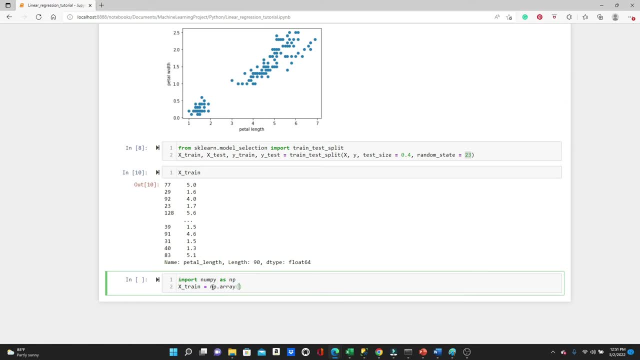 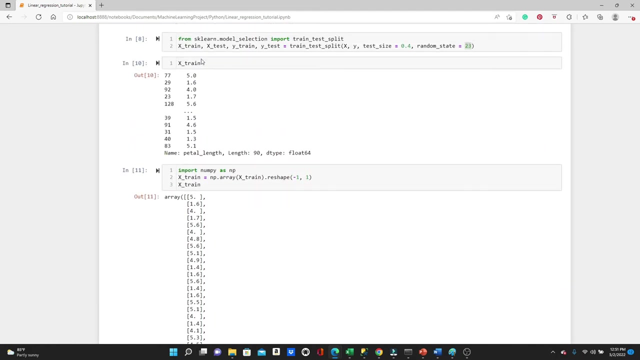 need to import numpy libraries first and then x train. we need to np dot array is to convert it to array. x train, dot reshape minus one one. now you can see here that the states are one-dimensional. look extreme, here it is. it's two-dimensional. now look at it, we are. 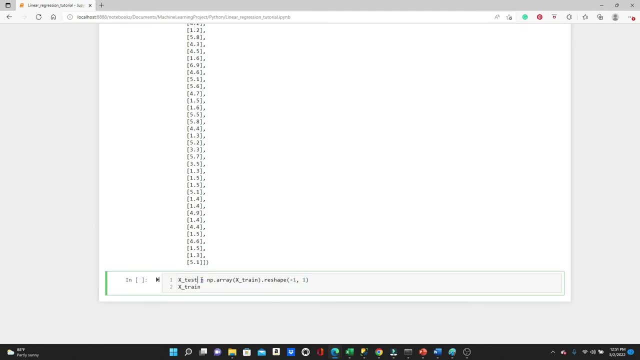 going to do the same with X test. okay, X test. X test became two-dimensional as well, so data is original. so we need to import the linear regression from scikit-learn library, first from scikit-learn dot linear model. import linear regression. now, let's say the linear regression model to a. 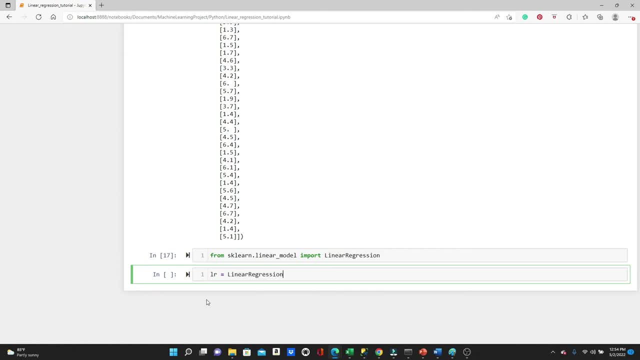 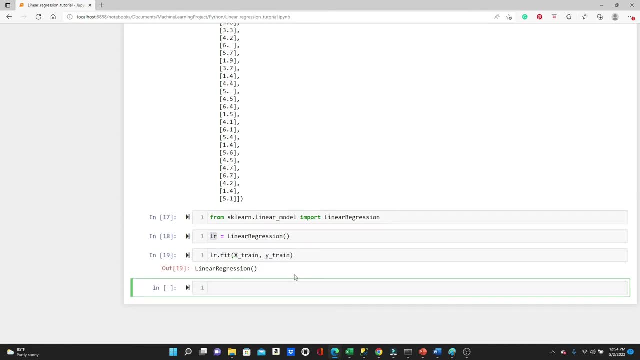 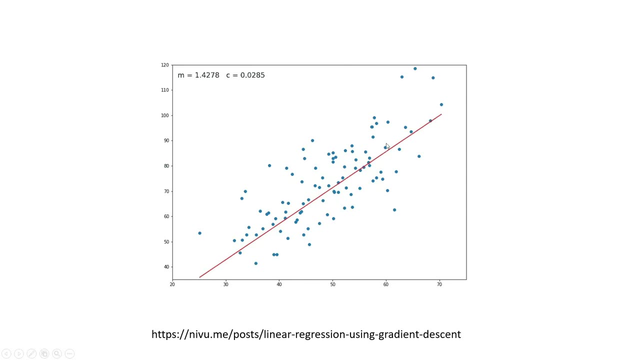 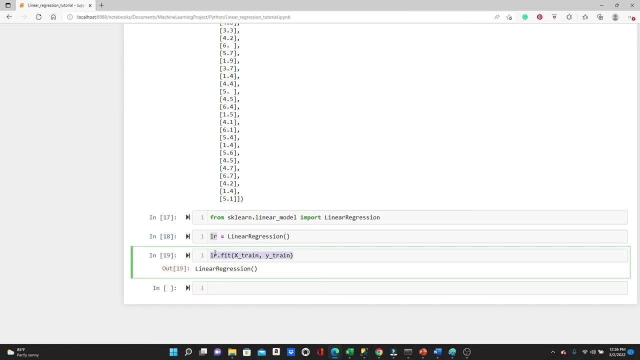 linear regression model for these will do. we talked about how we keep changing M and T and we find the optimum M and C for this best fit line. to fit this straight into the dots, when we fit X crane and Y crane to the linear regression model, this is one of the most productive regression model, far to the. 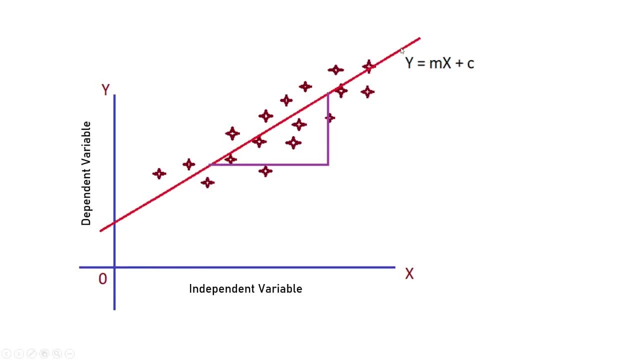 is what happens. it finds this m and c to find this best fit line. generally m is called the slope of the line and c is the intercept right. but in machine learning m is called the coefficient and m and c are called the training parameters. when we fit x train and y train to this linear 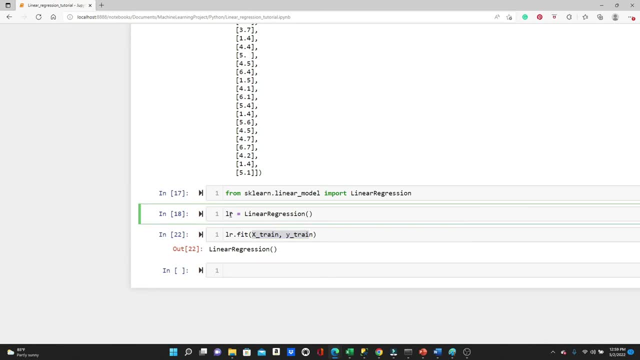 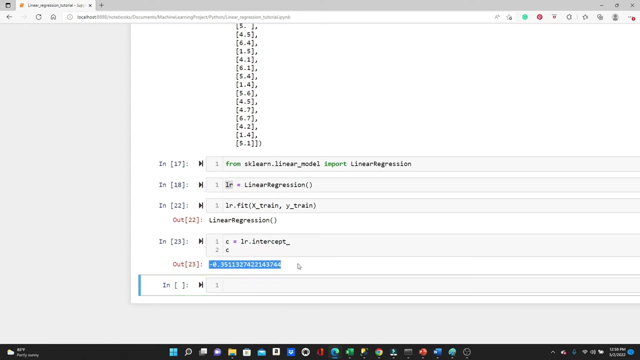 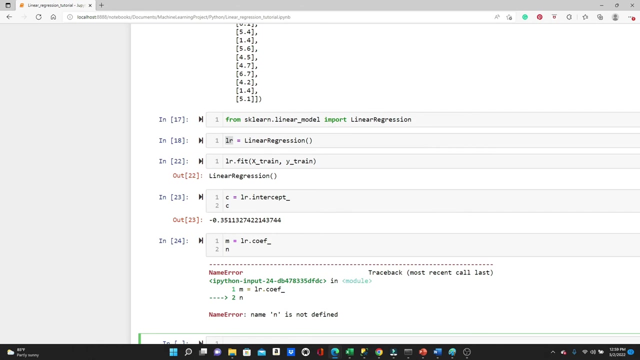 regression model. this is called the training. that means we actually trained this model and after this fitting process is done, that means the training is done. this lr model should have the training parameters m and c. okay, let's see lr dot intercept. so we have the intercept and look at the coefficient: lr dot 12 m or not m. 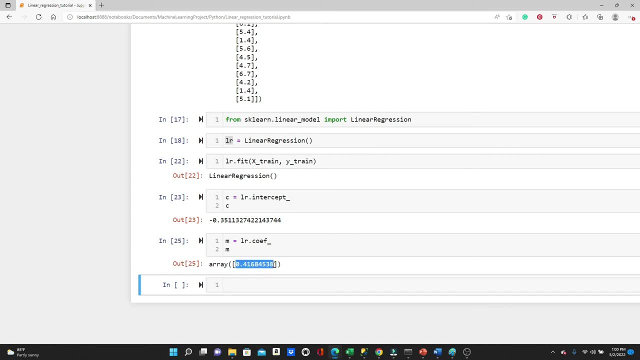 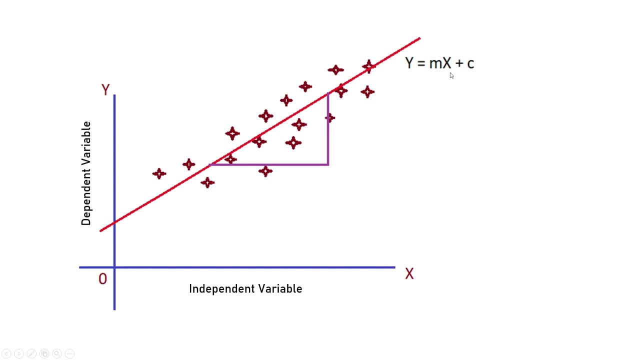 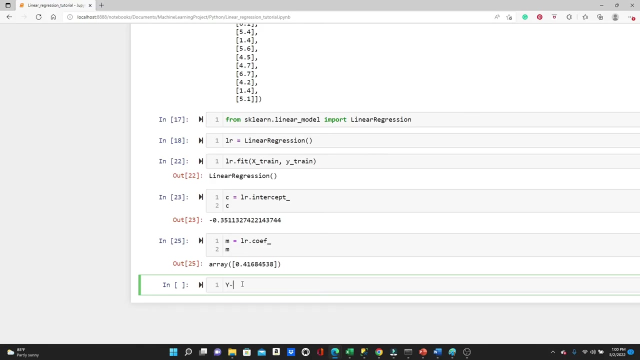 yes, this is the m, the coefficient or the slope for the linear model. now we already have m and c. so if we have the x now we should be able to estimate the y. let's see if we can estimate the y y, crad crane. so first we take m. 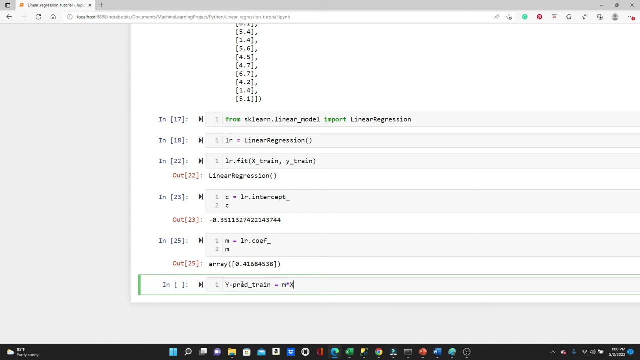 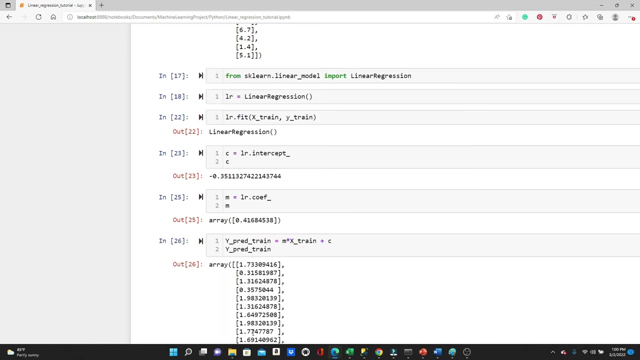 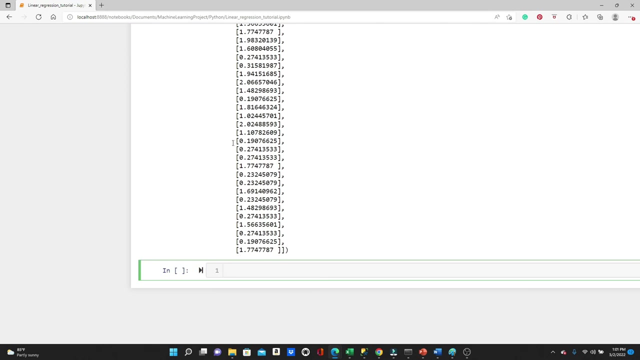 times m, times x crane plus c. so okay, instead of this let's put under score y red frame. so this is how it looks like. okay, but for scikit-learn library there is a predict formula, so you can use directly the predict formula. lr dot, predict x crane. we already fit. 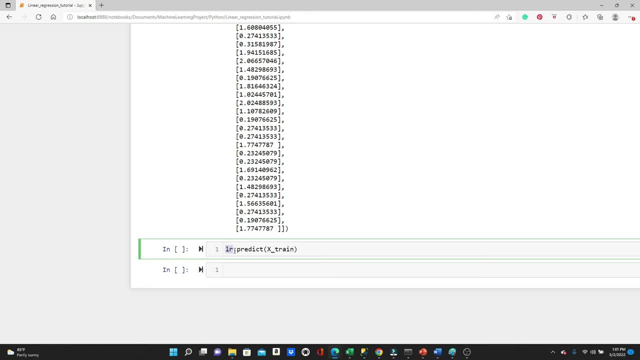 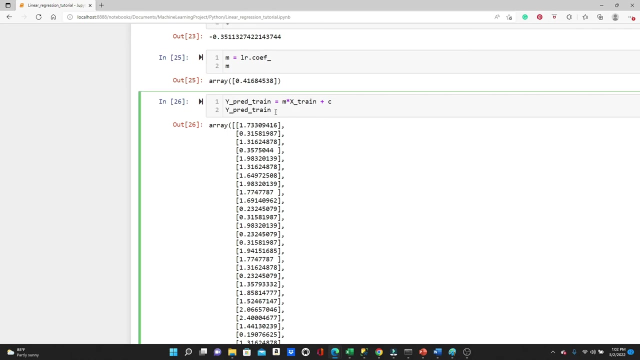 x crane and y train to the lr. that means lr should be trained and it should be able to predict. now, okay, let's do it. y red frame 1. now, y red frame 1. you can see here. okay, I will flatten it. okay. so this one is one dimensional. so let's make this one one dimensional too. so, 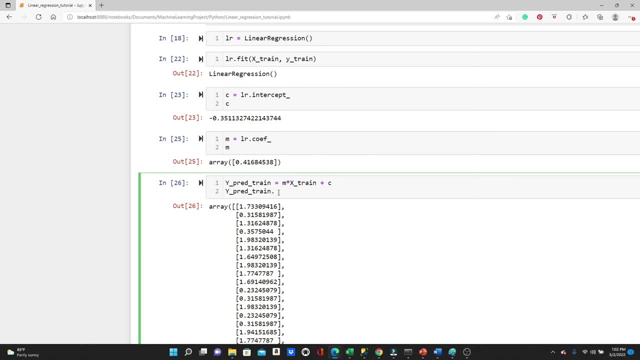 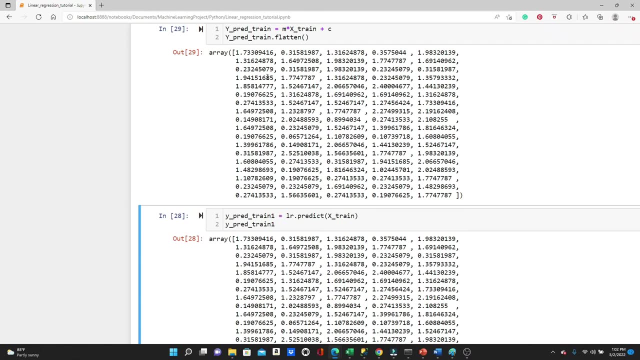 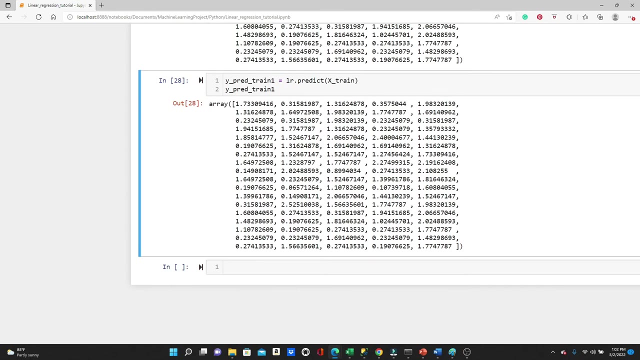 that we can compare dot flatten, so it will become one dimensional. so you can see that the values are exactly the same. one point seven, three zero point three. one five. one point seven, three, zero point three. one five. one point nine eight. one point nine eight. so these are exactly the same thing. so you do not. 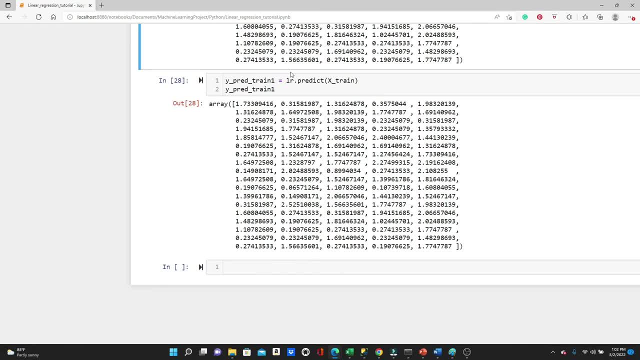 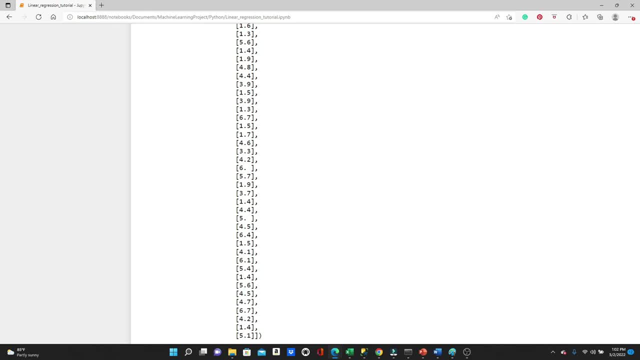 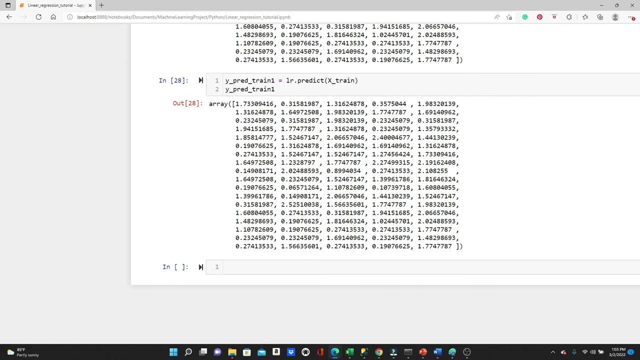 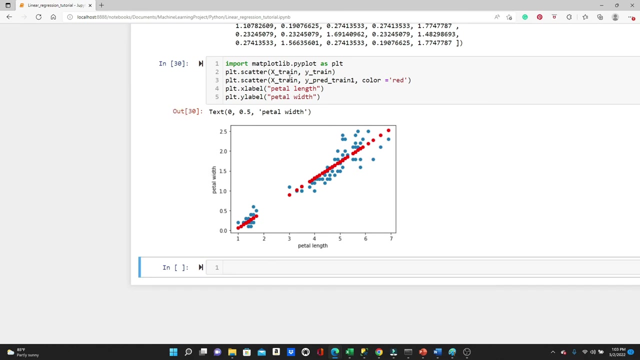 need to calculate like this. you can simply use the predict function and it will calculate it for you. let's check if we found the best fit line. okay, let's just copy this and paste it here: this prediction. now see, we found our best fit line. this is the red line. this: 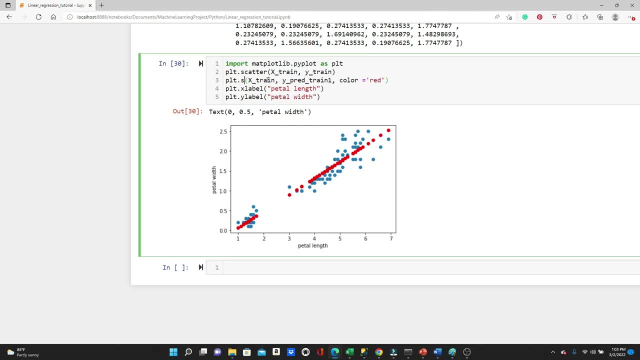 is the best fit line, isn't it? instead, we can actually put the line. now. if we have the pedal length, using the model, we can actually get the pedal width, even if the pedal width is not directly on the dot, but at least it will be close enough. 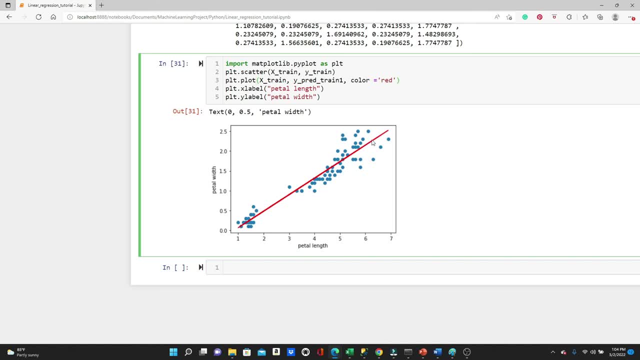 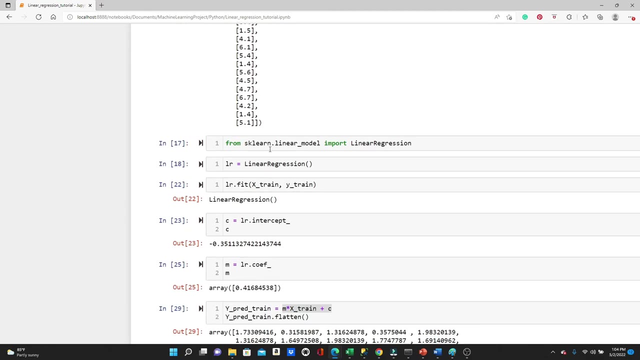 isn't it? if it's here, at least we'll find the value here. so it's going to be at least close enough. we used x-train and y-train all this time. now what to do with x-test and y-test? we used x-train and y-train to train the model right. 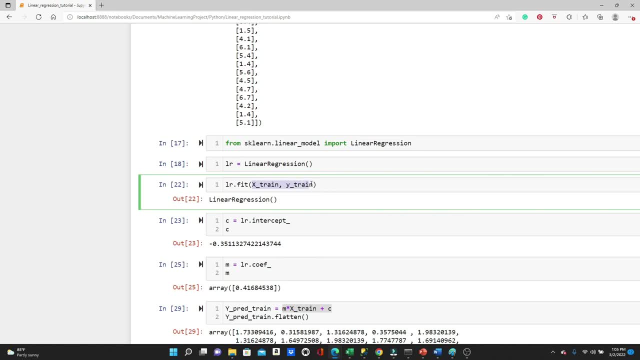 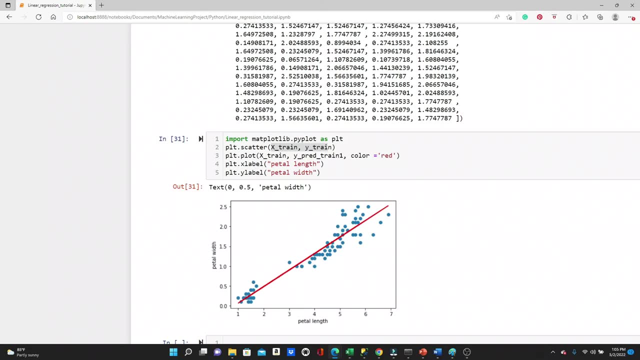 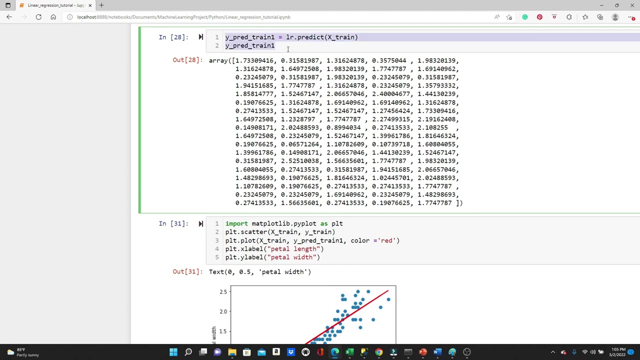 here. but the model have never seen x-test and y-test, so we can test this model using x-test. now let's see the way it was able to predict for x-train, if it can predict the same for x-test. so let's copy this and: